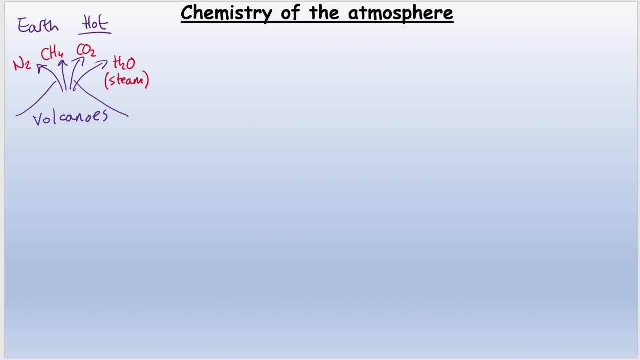 so for Mars, Venus, for example. Now, because those gases were all up in the atmosphere, what happened was that formed the greenhouse effect and that contributed to the increasing, or the increased, temperature at the time. Now the greenhouse effect. we're going to just quickly go through to make sure that we all understand what we're referring to. 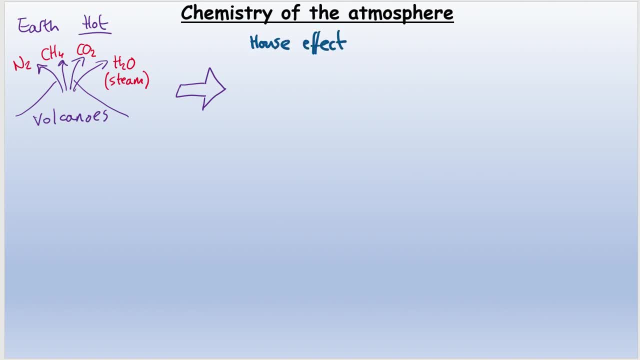 when we talk about it. Now, the greenhouse effect is where you've got the earth and surrounding the earth. you then have your atmosphere. Now this is the atmosphere, and then you've got the gases that are building up within it. Now what would normally happen is: 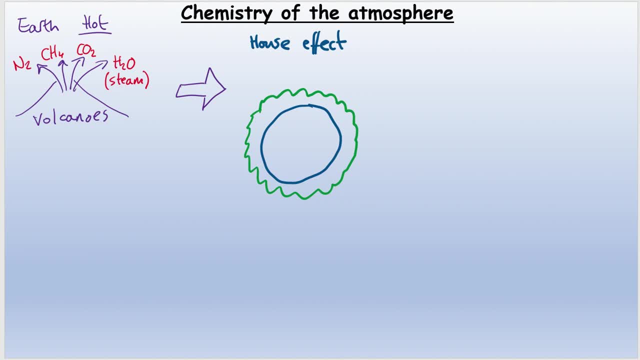 infrared radiation, so heat radiation from the sun would come in and it would be coming through and some of it would be absorbed into the earth, okay, and then, as it would then leave, some of it would get out and escape Now the problem with greenhouse gases. 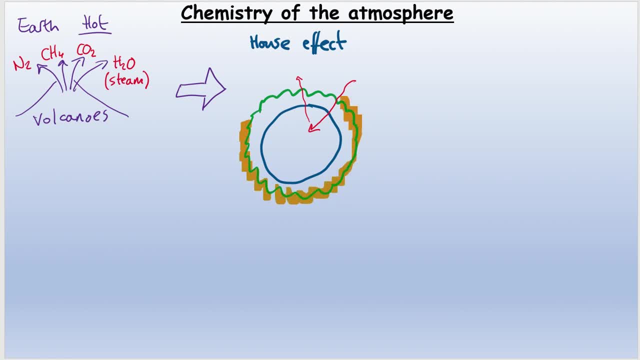 is that they build up a layer in the atmosphere. that means that as the heat or the infrared radiation goes to leave, it can't. and what happens is it gets trapped in this layer and this layer gets warm and then radiates that heat back down. and then it gets trapped in this layer and this layer gets warm and then radiates that heat back down. 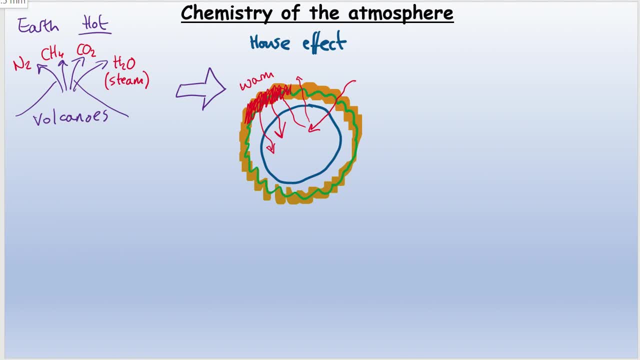 and so, because it's radiating that heat back down, the earth then gets warmer. It's important to remember that. the greenhouse effect- I've just noticed I've not done that up there- the greenhouse effect okay- is a good thing. it's what makes our planet. 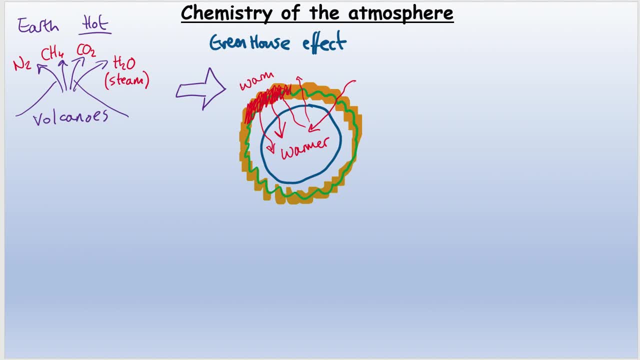 at the moment inhabitable. it's what keeps us warm. It's the enhanced greenhouse effect that you hear about a lot in the media, where they refer to the fact that obviously we're contributing to the enhanced greenhouse effect which is leading to global warming, etcetera. 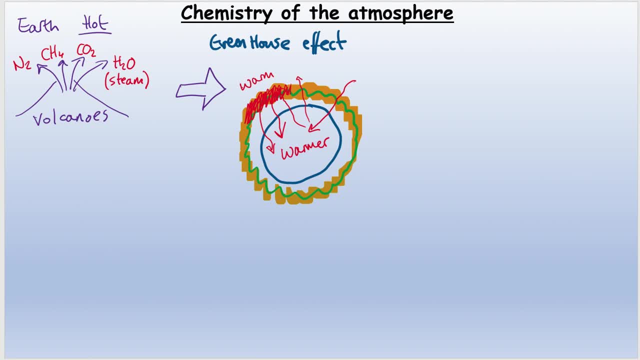 What happened was, over time, the earth then slowly began to cool down, and as it began to cool, what that meant was that the water that existed at the time- so that's my water- I've got in its steam form- it was able to then condense. 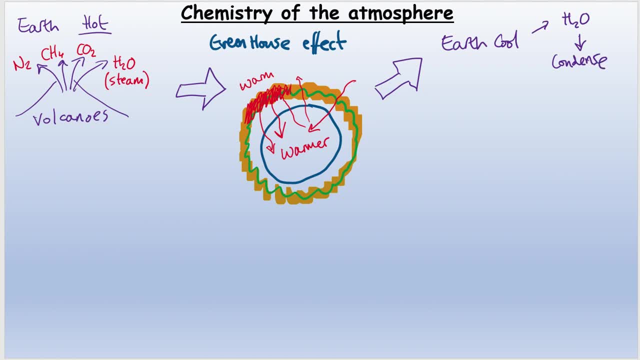 When i sayistical condense, I'm referring to the fact that it's changing from a gas into a liquid, to a going from steam into liquid gas, into liquid, into liquid water. As it then condensed, that meant that we then formed the oceans, okay, And 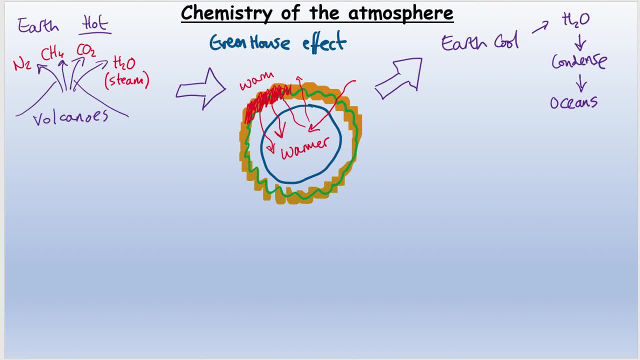 the oceans at that time because we had a huge amount of carbon dioxide. some of that carbon dioxide then dissolved into the oceans, And that meant that there was a slight decrease in carbon dioxide levels. Now, what then happened was that, because water was now available in liquid form, 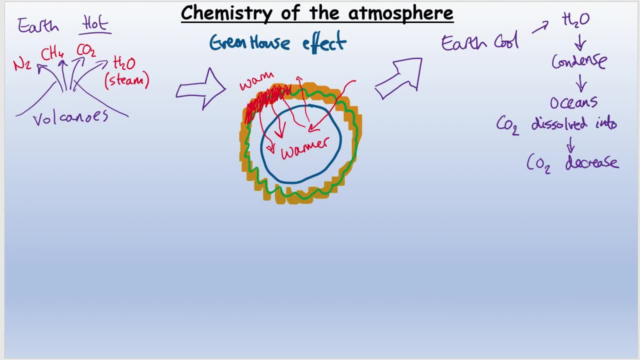 okay, around sort of 2.7 billion years ago, we then started to have algae form. Now, algae was a very basic form of plant life, And because it existed, it meant that photosynthesis could start happening, And so we then started to have algae form. Now, algae was a very basic form of. 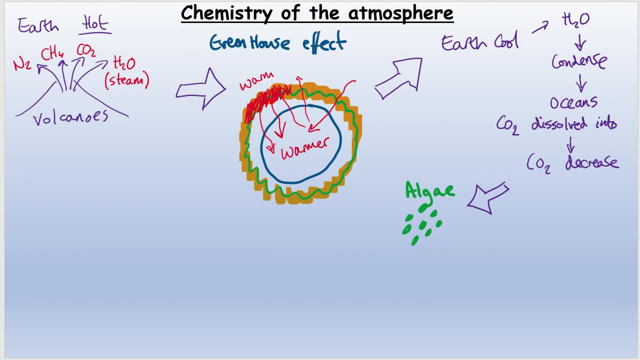 about sort of the next billion years after that. you also had then just your normal sort of plants that we think about now. okay, So less more complex types of plants. green plants then also began to form. So because they formed, they then led to photosynthesis- Now photosynthesis. 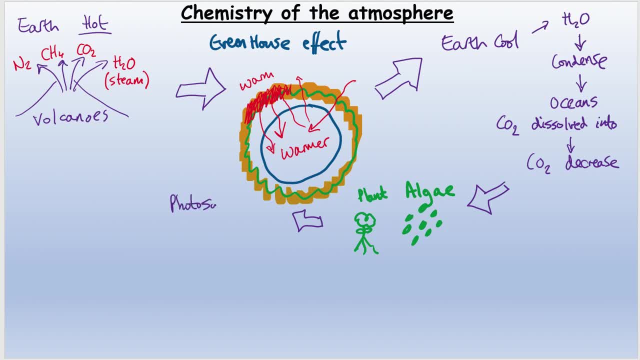 so we're going to come up here somewhere photosynthesis. Photosynthesis is the process whereby carbon dioxide- carbon dioxide- is reacting with water in the presence of sunlight and it's then forming glucose and it's forming oxygen, And it was the key thing here: it's this oxygen that's being formed. that then sort of really. 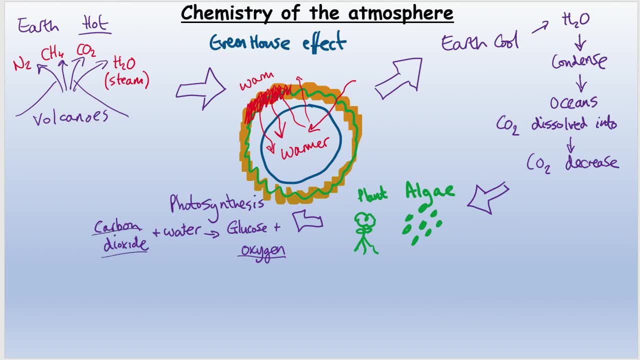 as well as the carbon dioxide being taken in, had the biggest effect on the Earth's atmosphere at that time. So what happened was all of that that was given off. okay, meant that the O2 levels, so the oxygen levels, increased, So they increased And at the same time, because the 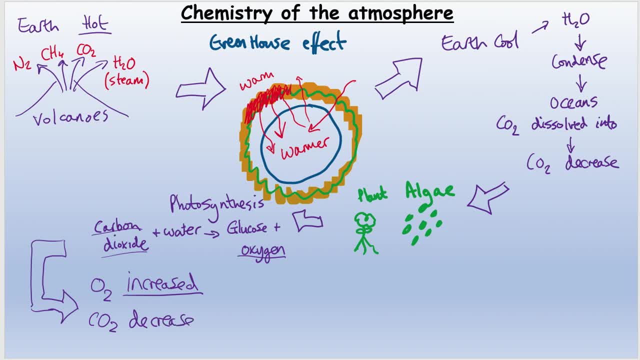 carbon dioxide was being taken in that then decreased Because we had an increase in the amount of oxygen level. that meant that things like animals, birds, fish, more complex life okay. so from the O2, we ended up with more complex life evolving. 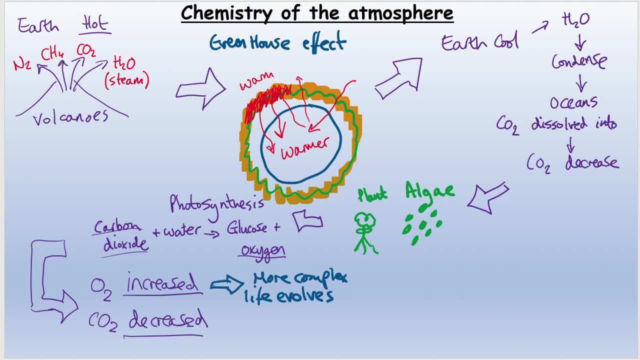 Now that complex life, if we were thinking about it as sort of spurring off and looking at something slightly different, that complex life then went on to form well, to die, and then form things like: so they die, Which then leads to things like fossil fuels being formed: Coal, oil, gas. 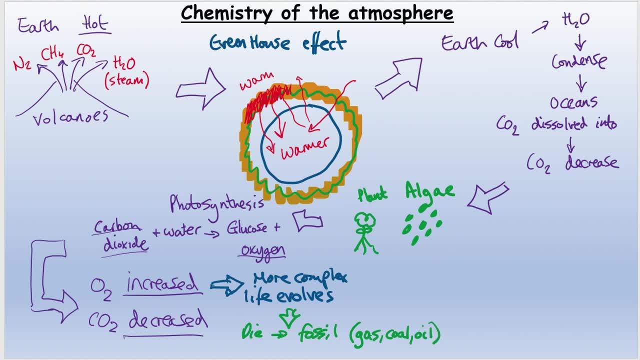 Now, as that all then happened sort of- if we think back about sort of 200 million years ago, we then ended up with an atmosphere that actually is almost relatively the same as our current atmosphere today. It hasn't hugely changed very much. 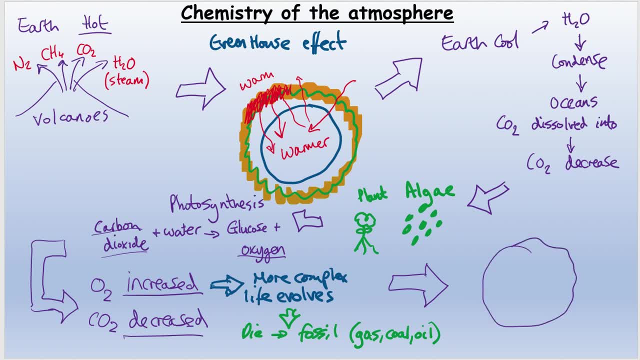 We ended up with an atmosphere that consisted of a large proportion- and we're talking around 80%, approximately 80%- of nitrogen. You then had approximately 20% of oxygen, and then you've got less than sort of 1% of just other gases, which are things like: 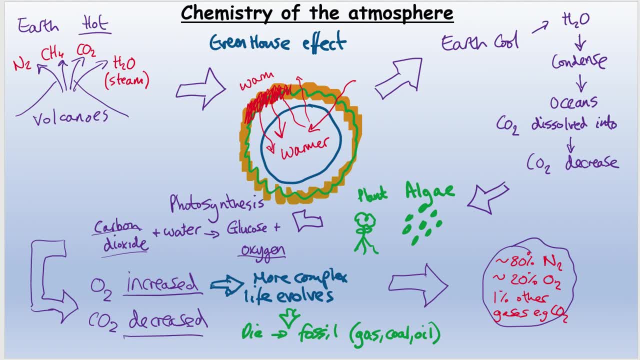 carbon dioxide, so EGCO2, okay, Now the nitrogen built up because it was originally being given off by the volcanoes, So we ended up with an atmosphere that consisted of a large proportion, and we're talking around 80%, approximately 80%, of nitrogen. 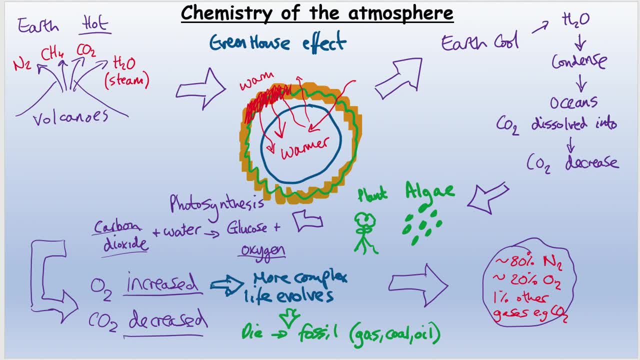 And it's relatively unreactive. It formed nitrogen-based compounds but a large proportion stayed as gas in the atmosphere. The oxygen built up to around 20% because of the photosynthesis. CO2 levels then significantly dropped again because of the photosynthesis and also because 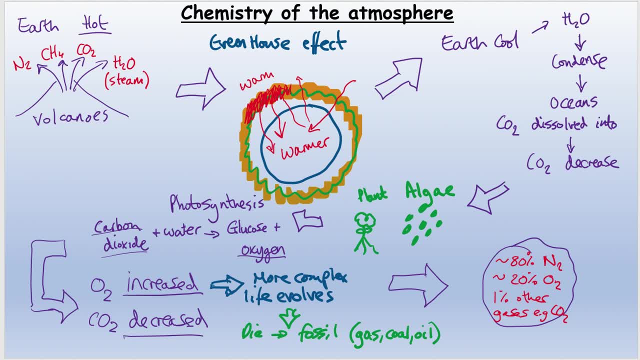 some of it was being locked away in the oceans of the world. That is kind of the whole of the chemistry of the atmosphere in a nutshell. Of course, in addition to this, there are other factors which have then led to our atmosphere slightly changing. in today's current atmosphere, That would be things like looking at combustion. 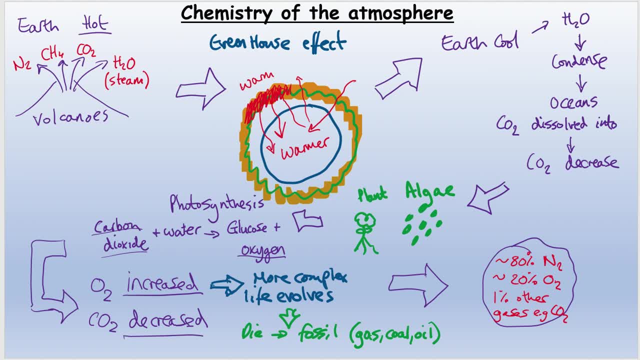 burning of fossil fuels, various things like that, which I'm going to do in a separate video, But that is the sort of the story. as we go on, We had a very hot Earth that had lots of volcanoes releasing those gases. That was all then contributing to the greenhouse effect. The Earth began to cool down. 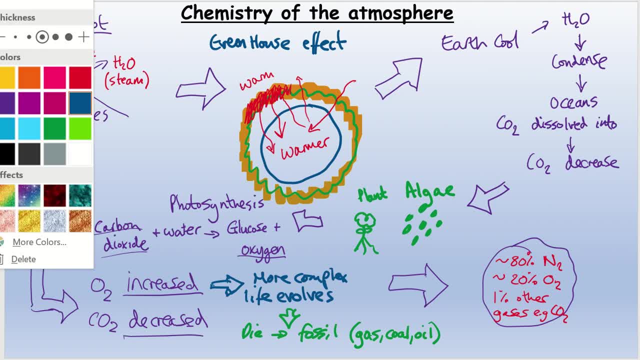 and it's important that you recognise that. So we had a very hot Earth that had lots of volcanoes releasing those gases. You recognise there that the Earth is cooling down at that stage. So the Earth gets colder and it's only because it gets colder that the water then condenses, forms the oceans.